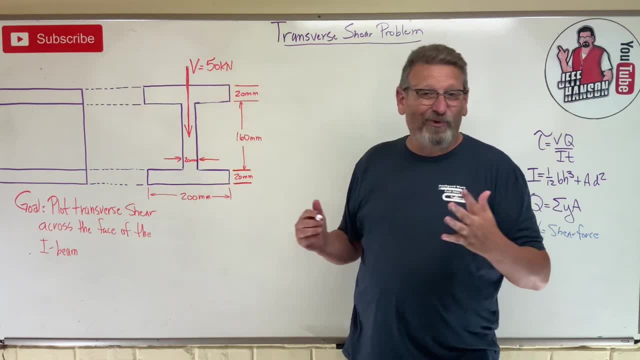 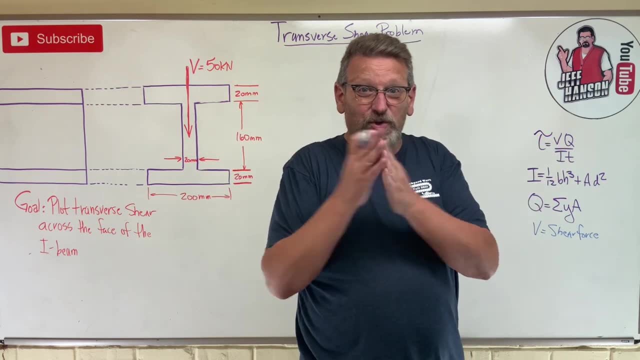 problem right, They just give you the shear force. Or another way- which is what I probably put on the test- would be to give you a beam And tell you to do the shear moment diagram And then go look at the biggest shear force on that. 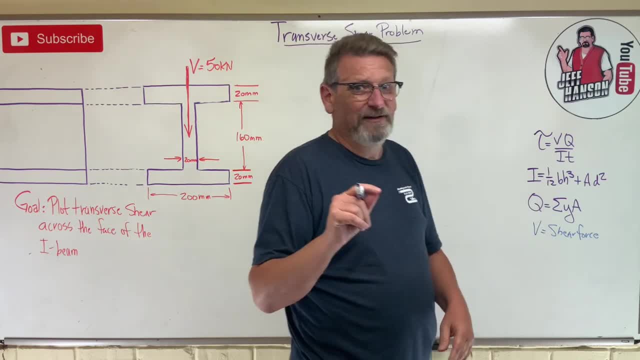 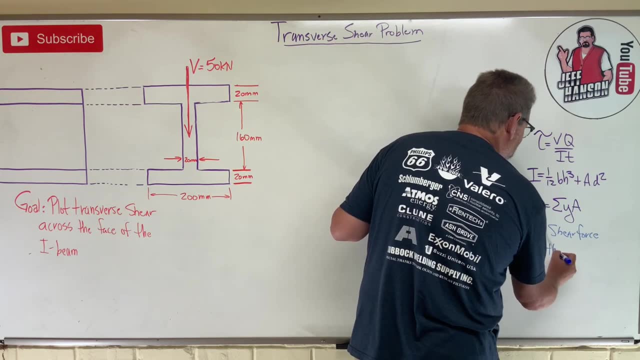 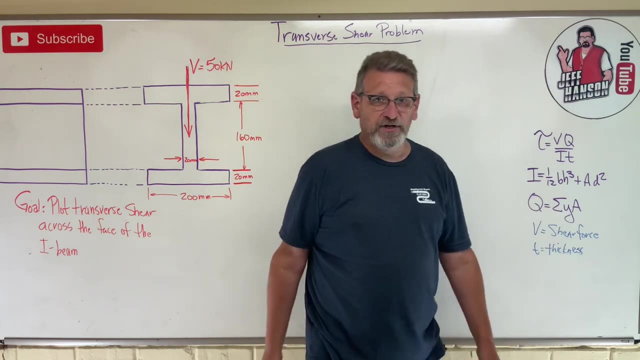 beam and use that for your V right. That would be even better for a test, wouldn't it? Okay, What is T? T is the thickness. Is that with two C's or one Q? Come on now. The thickness of the. 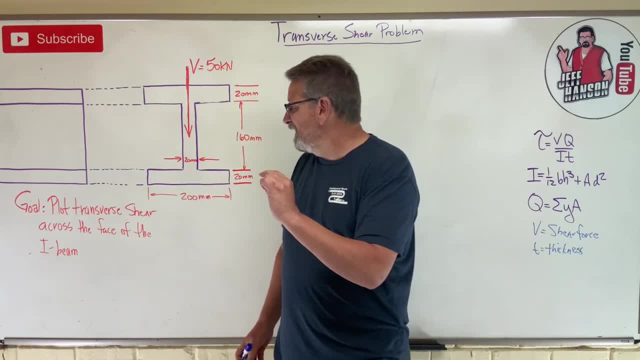 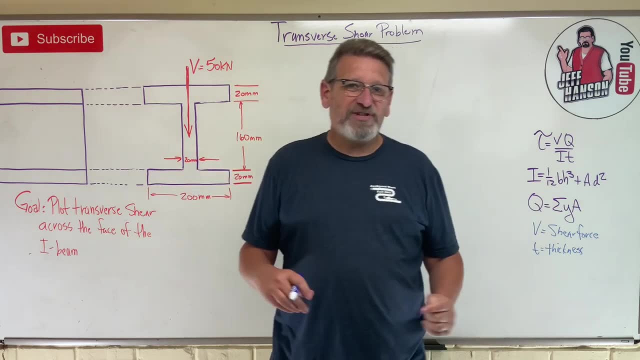 beam at the point of interest. Wherever you're trying to find the thickness of the beam, you're trying to find the thickness of the beam. So in this part the thickness would be 20.. In this part the thickness would be 200.. So T is just the thickness of the beam. Think, if I have to shear. 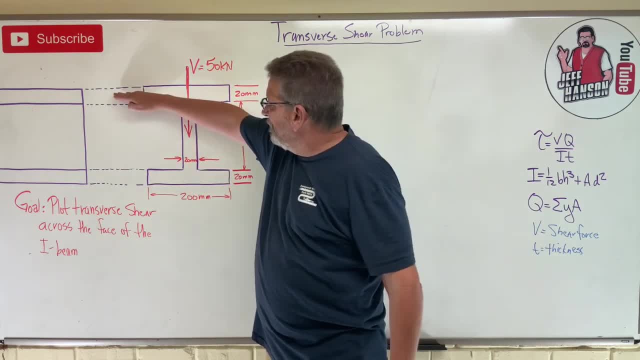 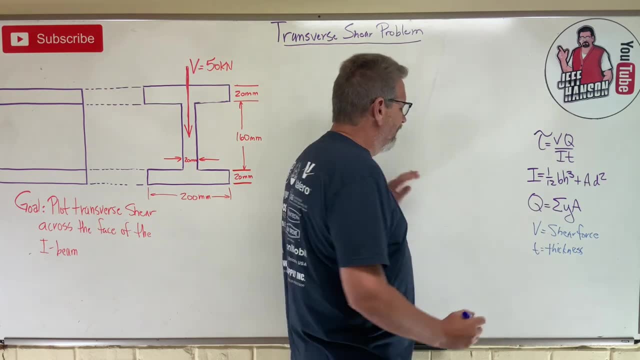 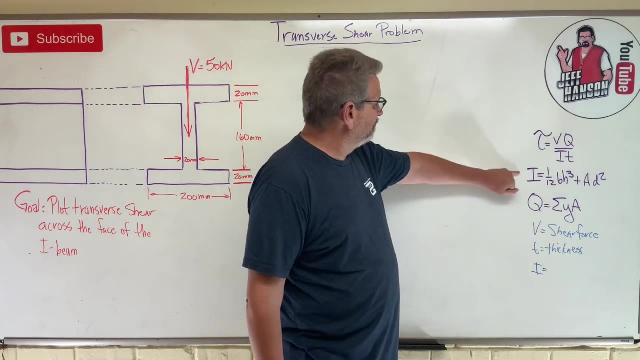 through that whole entire plane. How much thickness am I going to have to shear through? Down here it's skinny Down there, up there it's fat, right, Okay, That's what T is. And then, of course, I. well, there's our old friend, the old second area: moment of inertia. That's how to. 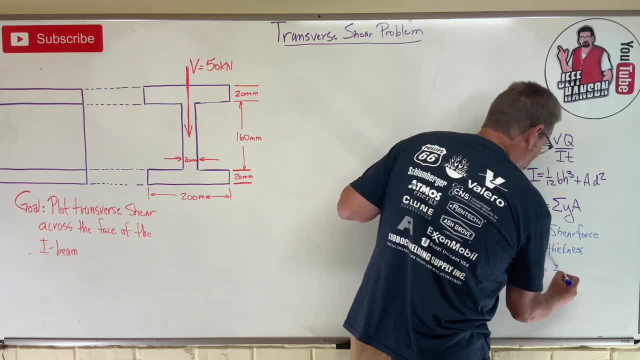 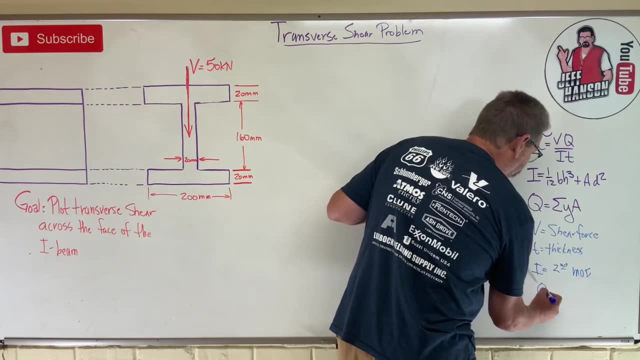 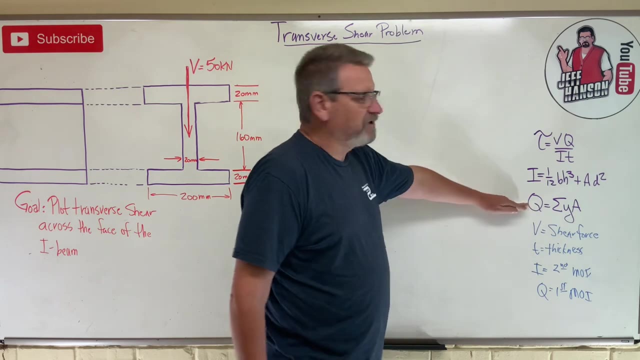 do that for rectangular beams. okay, This is the second. We'll put MOI for moment of inertia And then, of course, Q, the first area moment of inertia. okay, And we talked about how to calculate Q in the last video. So if you're lost on that, go back one video and you'll be golden, okay. 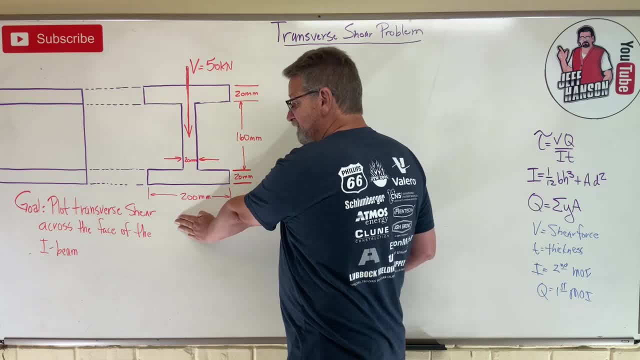 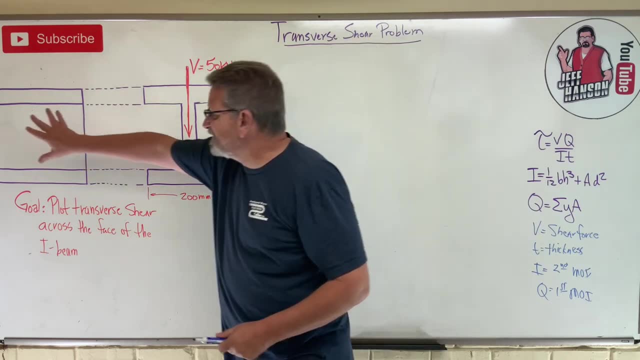 So what they want us to do here is plot the transverse shear across the face of the beam. Now, this is like an end view. This is the end view of the I-beam. This over here is the side view. So this is what you would. 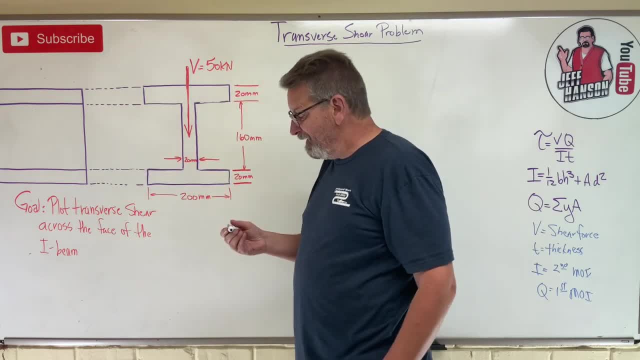 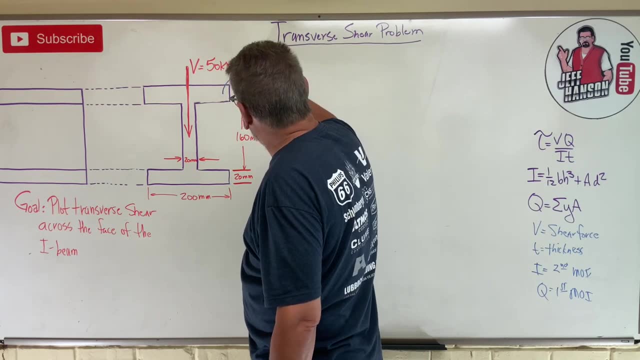 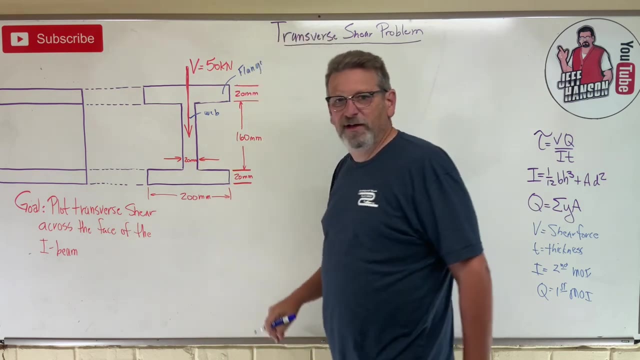 see, if you looked at it straight on that way, okay, And you remember about, do you remember about I-beams? What's this up here called? That's called a flange, okay. And then this part in here is called the web. okay, Just for terminology. So you sound smart next time you go on the job site. 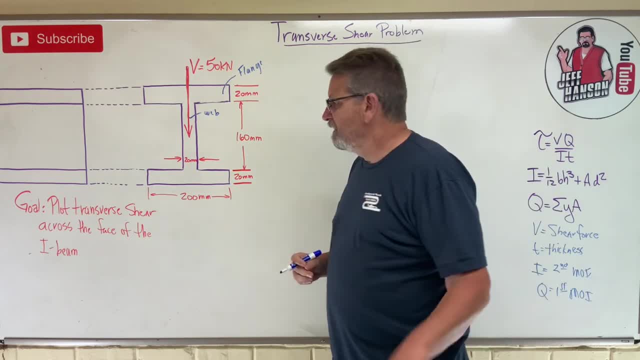 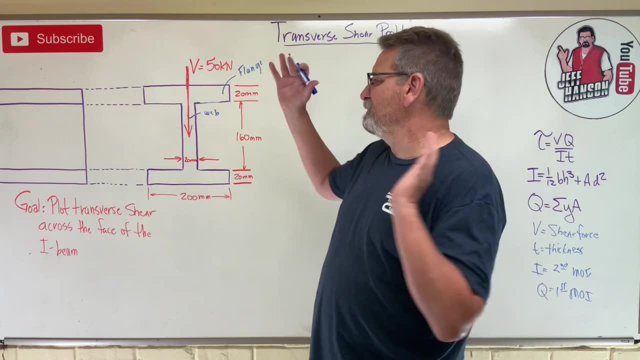 you'd be like: oh, that's a nice flange, you got on your beam there, okay. So step one on this is: you've got to determine where the neutral axis is. Now, this one is beautiful because it's a symmetric beam, The. 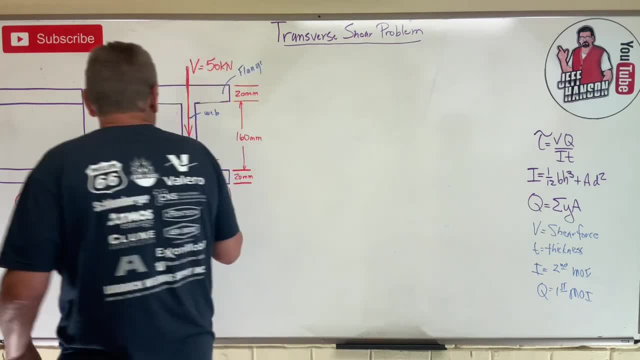 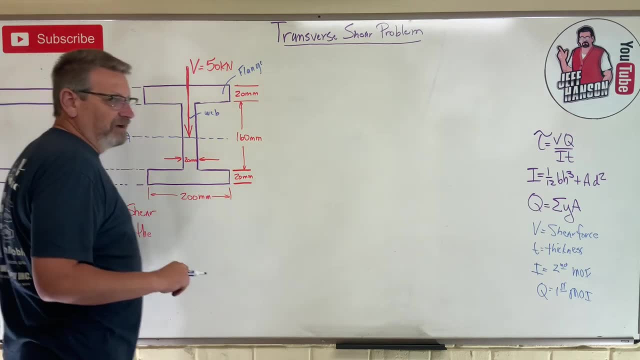 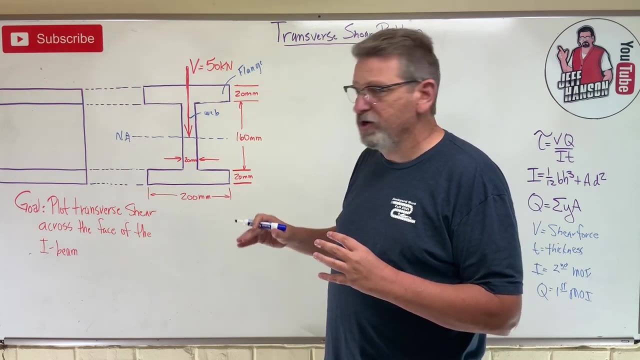 neutral axis is? it's apparent to me it's right in the middle. okay, There's the neutral axis. We've got to love symmetric beams, right. Okay, now for doing this, we're going to have to plot transverse shear. We've got to plot it. 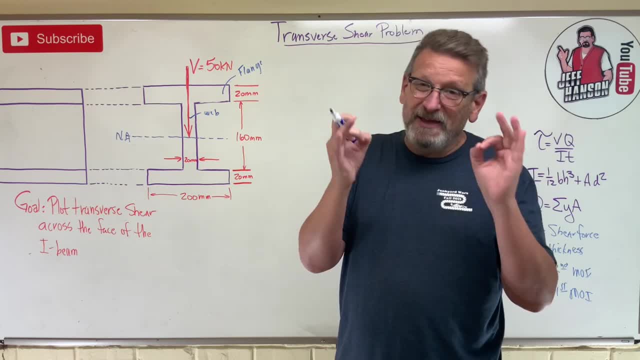 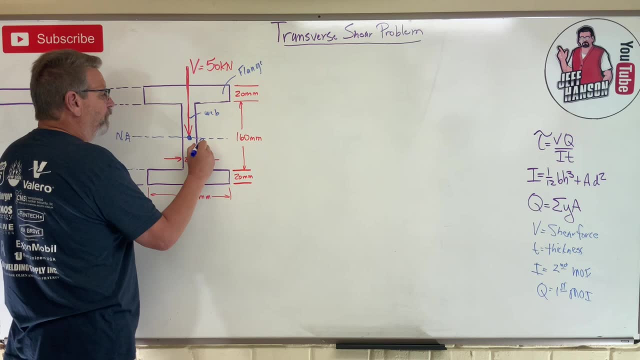 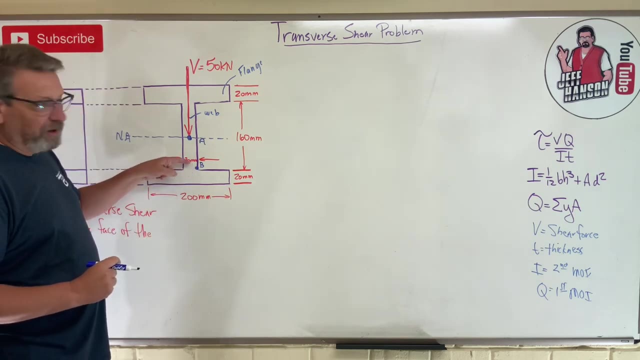 Several places to kind of get some key dimensions, some key points, okay. So I think one of the keys is going to be right here, okay, In the middle, I'll call that point A. I think, right here, okay, I'll call that point B. Now, point B is one molecule into the flange, and then I'll call this: 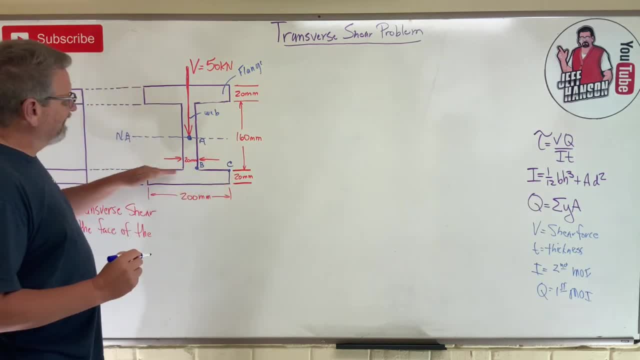 over here. point C: right? So this is in the flange and then I'll call this point down here on the bottom. point D: okay, And if we can find those one, two, three, four points, we can find this. I think we can plot. 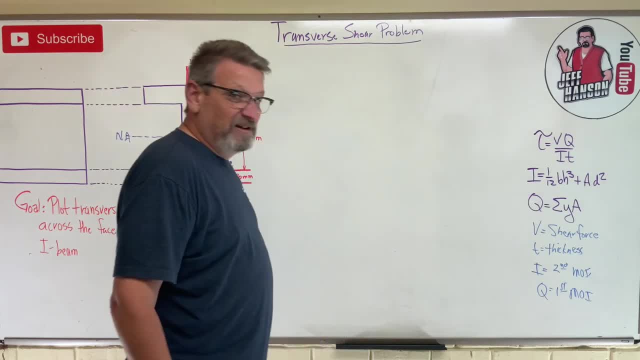 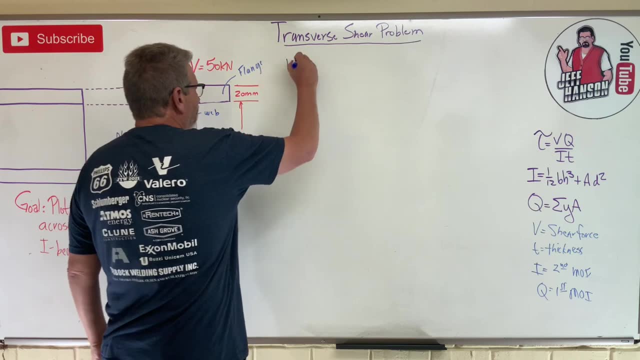 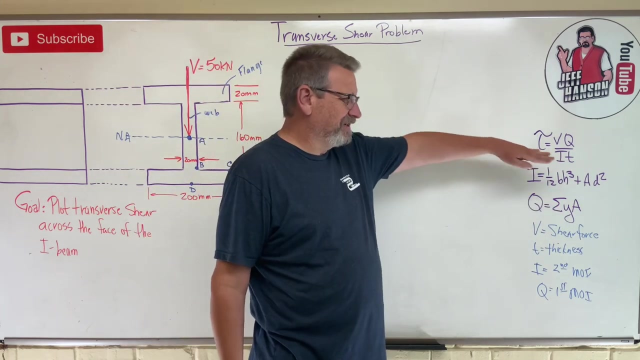 the shear for the whole entire beam. okay, Let's see if we can do it, Let's find something that. what do I have in that equation that works for everybody? Well, V, that's known. It's 50 kilonewtons. And I'm going to tell you- I've told you this 63 times- here comes 64.. 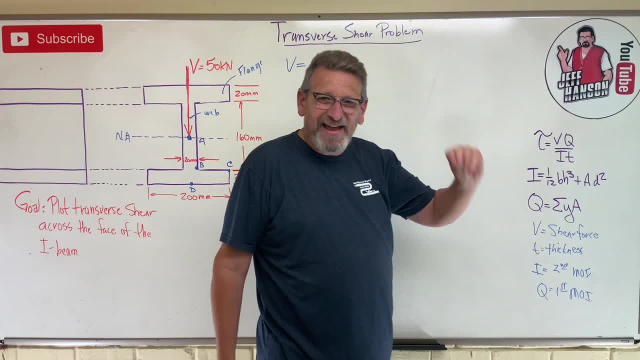 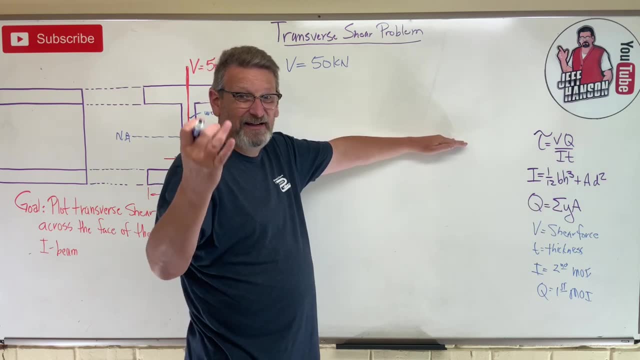 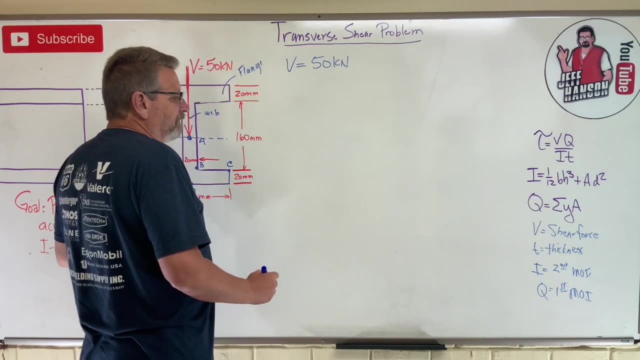 When you get a bunch of unknowns in here, make sure you're unit. It's all crossed out, right, Because what should tau be in? It should be in like PSI, KSI, PA, MPA, right, It's the unit of stress. okay, Let's calculate I, because I don't care what. 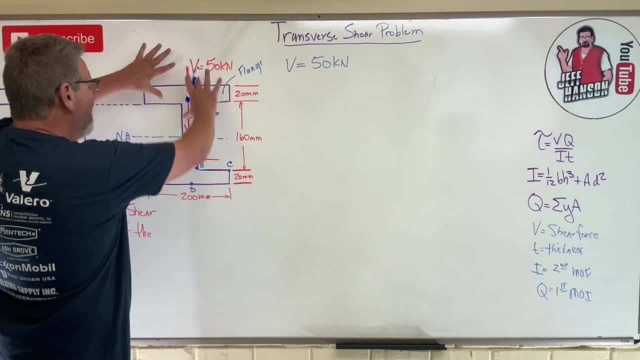 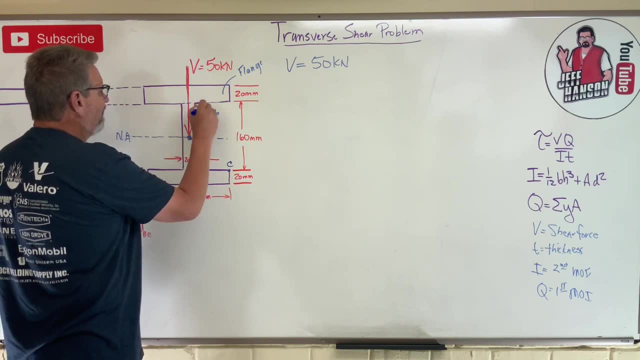 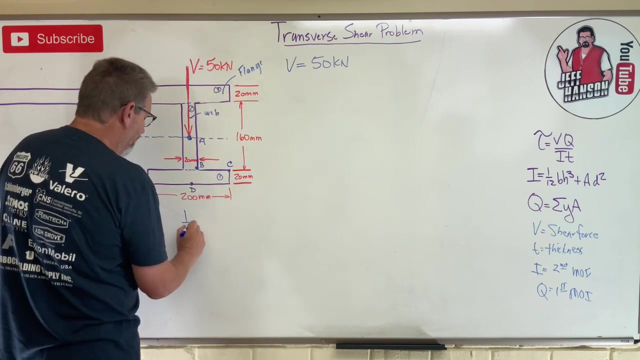 point I'm interested in. I never changes. I always is the I for the whole entire beam. okay, So what I'm going to do is this: I'm going to make him piece number one, piece number two, piece number three. So here we go. I is equal to 1, 12th, the base of piece number one, 200,. 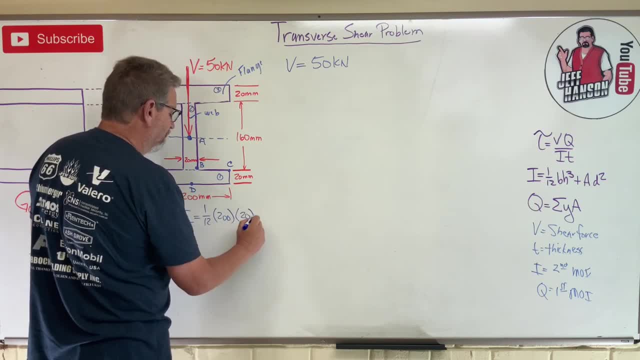 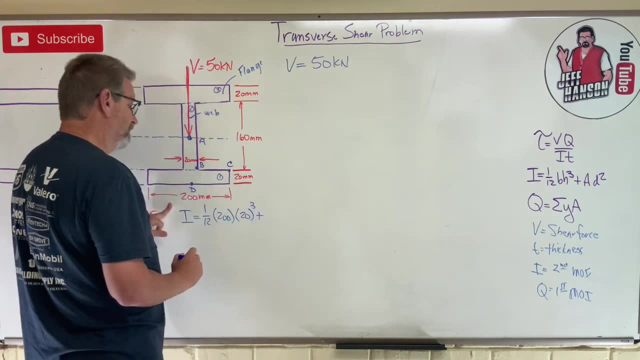 okay, The height of piece number one: 20,. okay, And that's cubed BH, cubed, right. There's our equation, right over there, plus the area, which is what? Four with one, two, three zeros, okay. 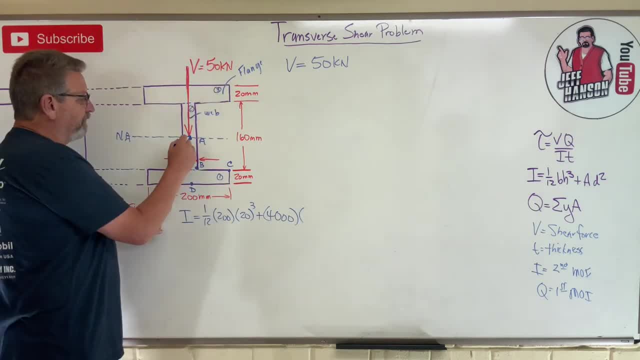 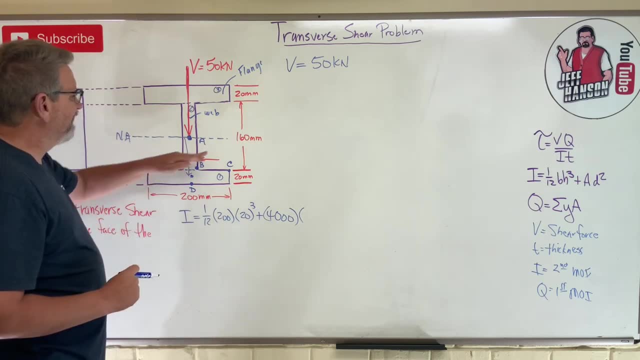 Times D squared Now. D is the distance from the neutral axis to the centroid of the piece, part right. So there's D right there. How far is that? It's 80 plus half of the 20, right, Which is 90, okay. 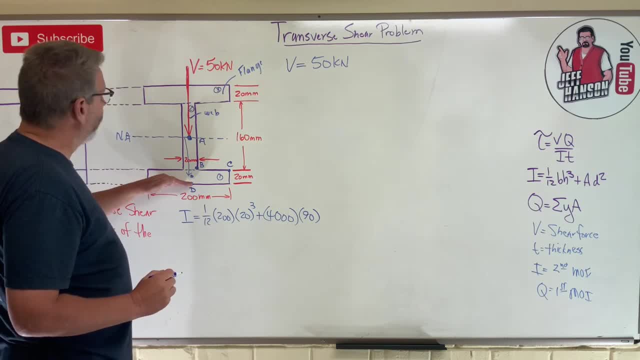 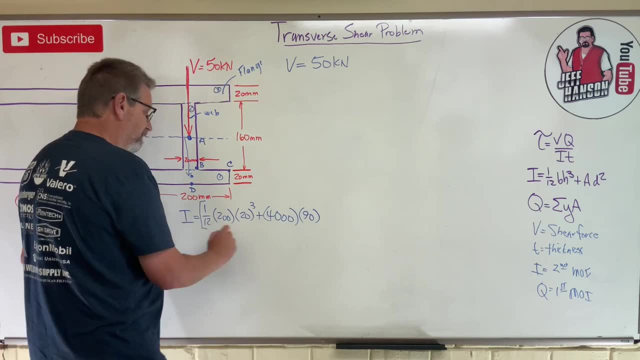 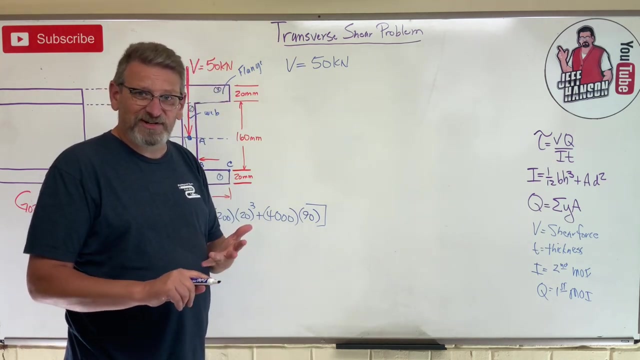 That's piece number one, Yo. what's different about piece number three? Nothing. So can we just tootums? that Did y'all learn your tootums in school. Tootums Like tootums two is four and tootums three is six. Y'all didn't learn your tootums. 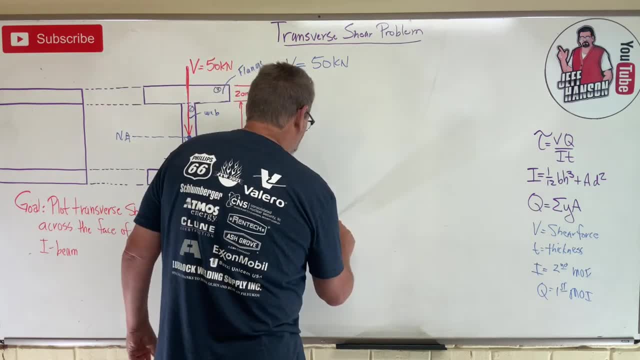 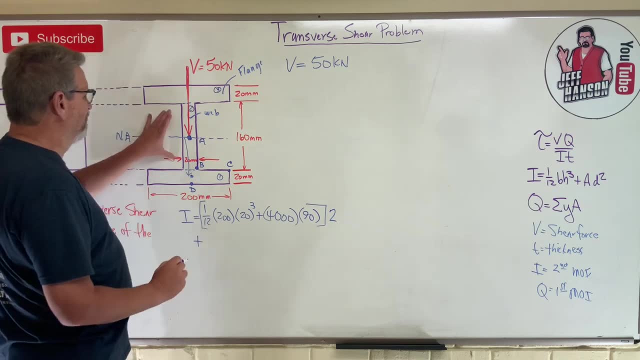 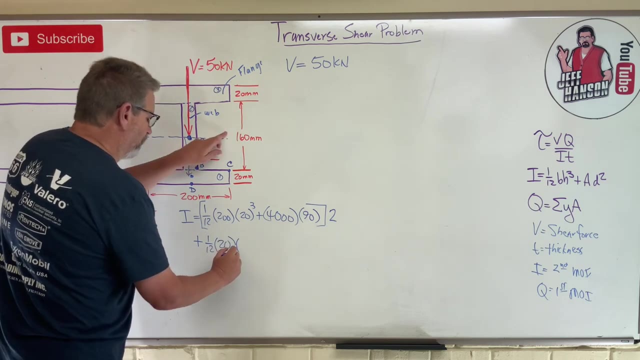 Okay, Maybe that's only in Texas. we do that. All right, So we'll put a times two on there, And then plus, here comes the second part. right, This middle guy is 1, 12th the base, which is 20, times the height, which is 160.. Now I don't have to do AD squared on this guy. 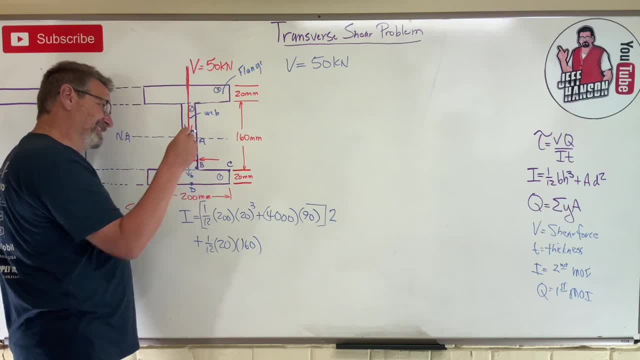 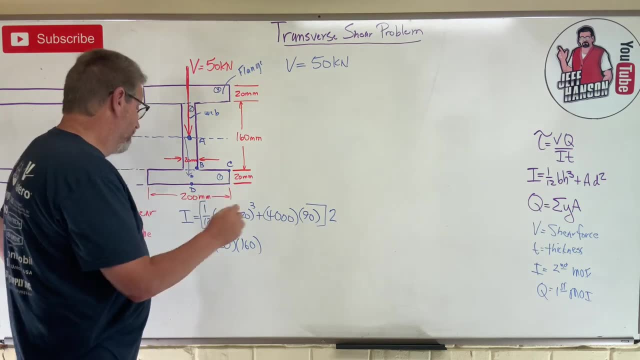 because what is D The distance? It's from the neutral axis to the centroid of part number two. The distance is it's zero. so that whole thing just goes away. So that's it right there. okay, Let's see if we can calculate. 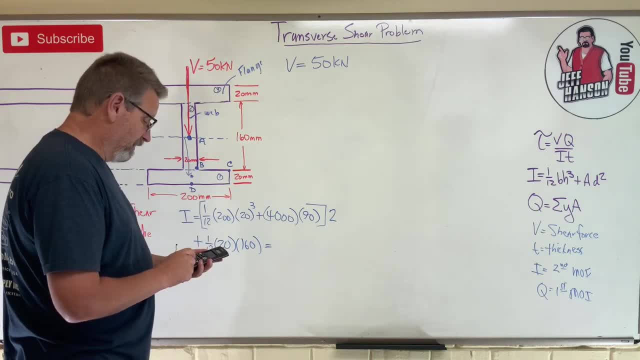 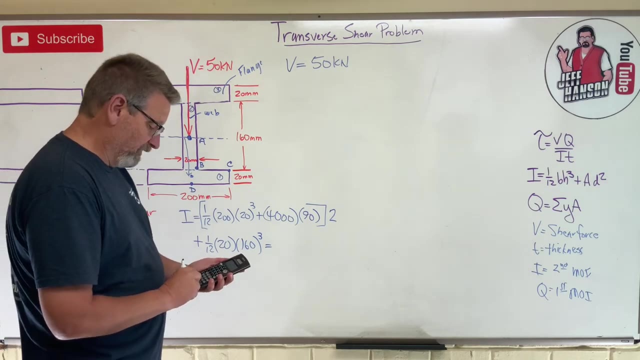 that, Come on handy dandy calculator. Let's go: 20 times 160 equals. oh wrong, I almost forgot that cube there, didn't I? That would have been bad news, wouldn't it? 20 times 160 cubed, and then divide it by 12.. All right, So I equals. this is a big number. 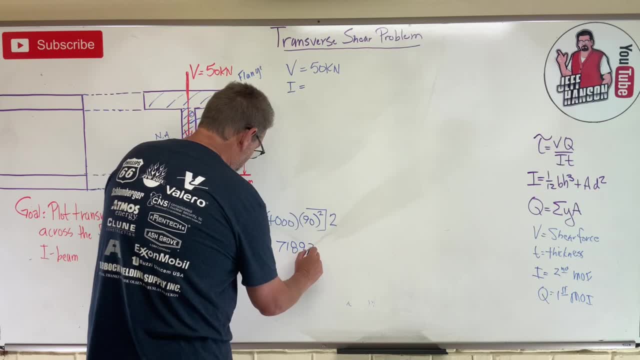 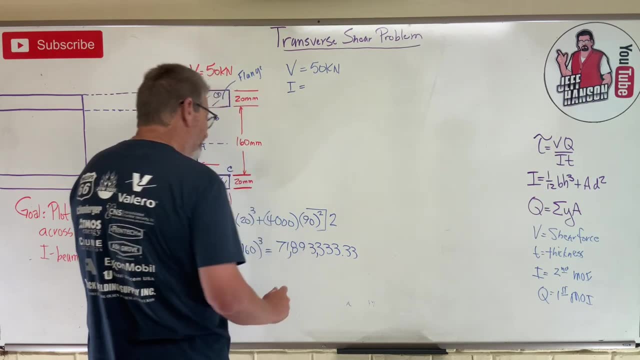 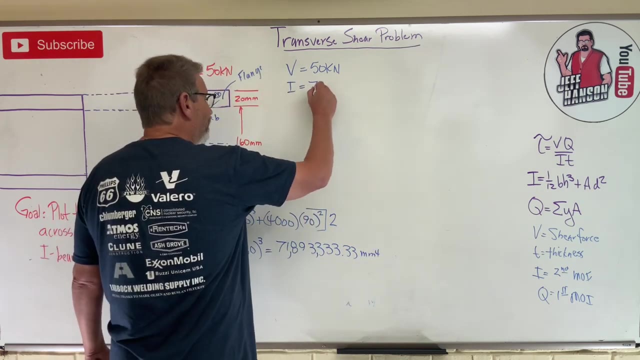 7, 1, 8, 9, 3, 3, 3, 3, .33.. Okay, But we're not scared of big numbers. Neither is your calculator. Now, that's I that's going to be in millimetres to the fourth. okay, So that I is not going to change. 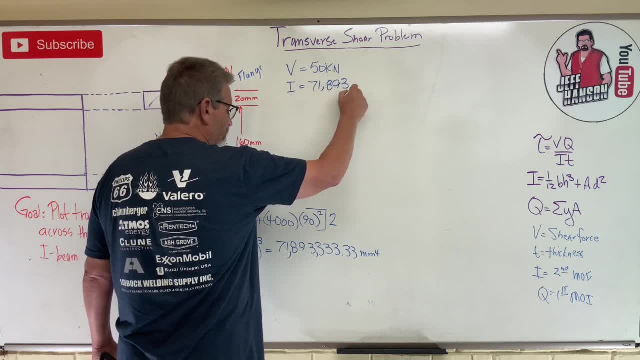 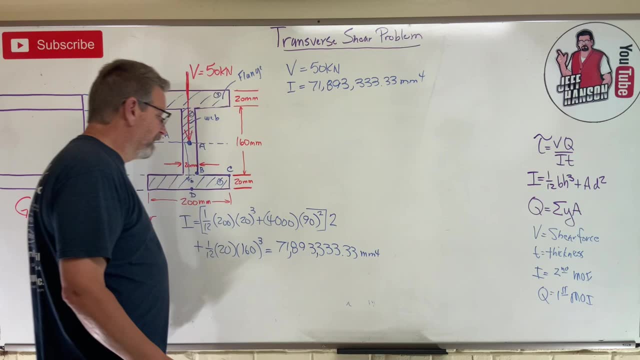 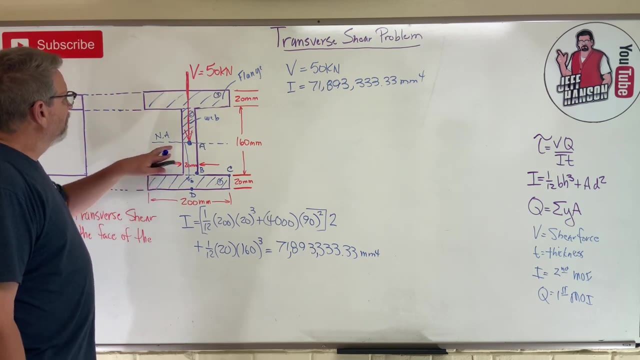 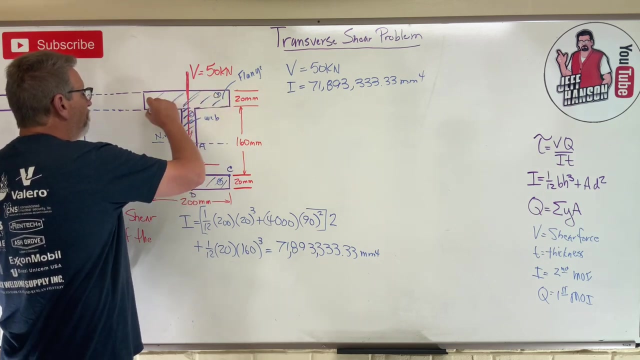 for any of the points that we're going to look at. okay, That never changes. Okay, Now what will change is Q. okay, Q will change. So let's find Q for point A. So Q for point A is going to be all of this shaded part here. I'm going to just do above the neutral axis, okay, So 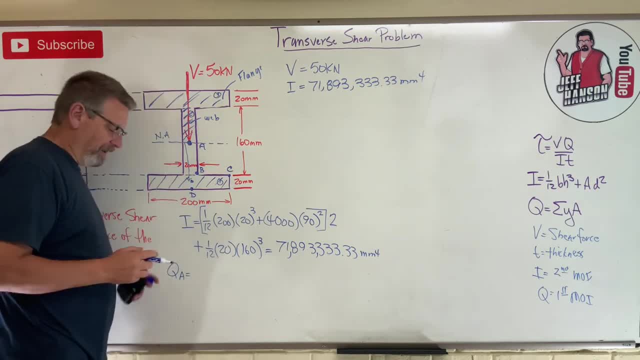 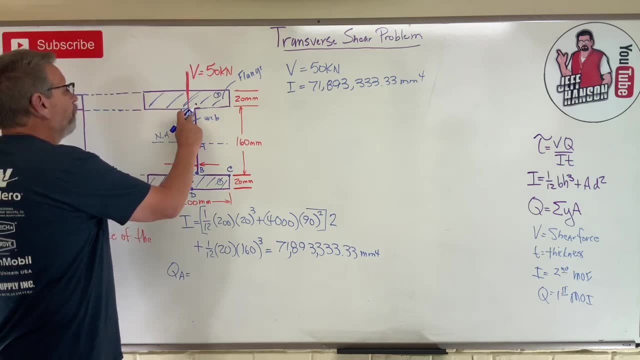 Q for point A equals- remember this comes from our last equation. so Q for point A equals. so Q for point A equals- remember this comes from our last equation. so Q for point A equals video. okay, Two shapes, So shape number. we'll make this shape number one here. Let's rearrange. 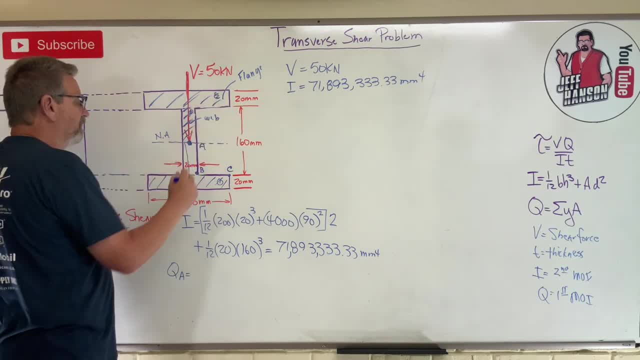 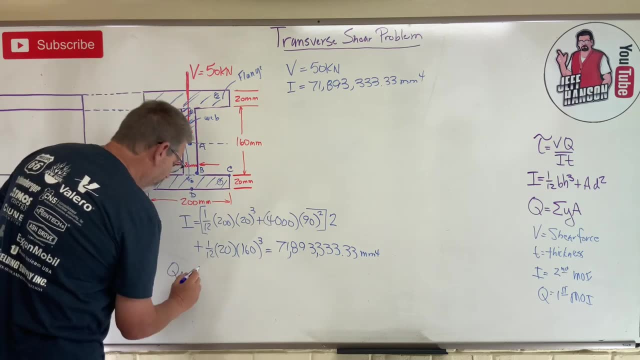 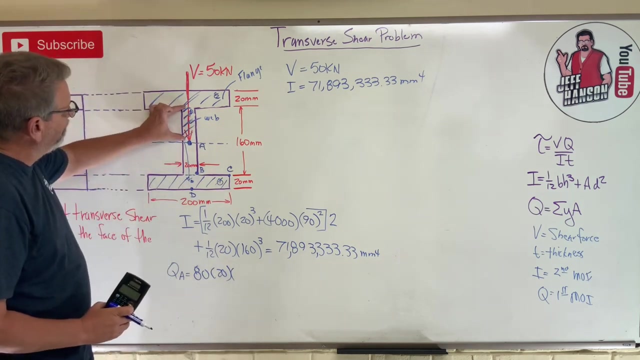 that, since we already did that, We'll make this one and then make that two. okay, So shape number one: the area is what? 80 times 20,? okay, 80 times 20 times. where is the centroid of that shape? 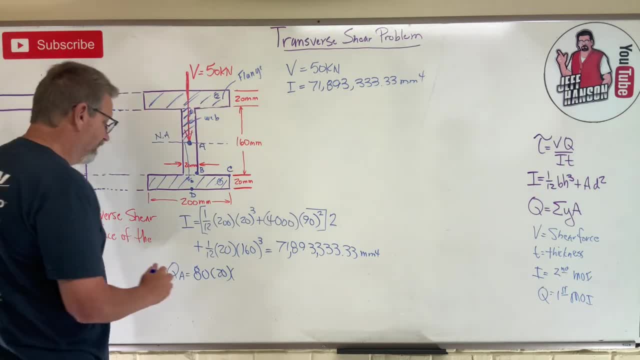 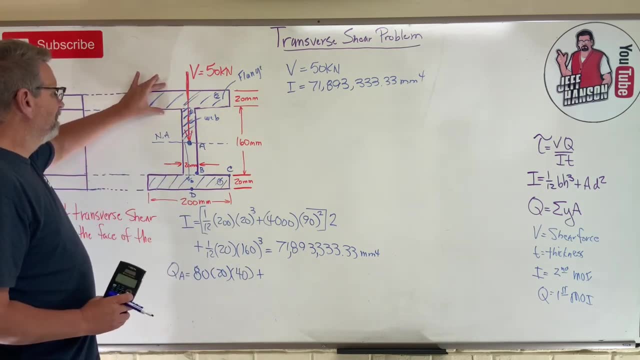 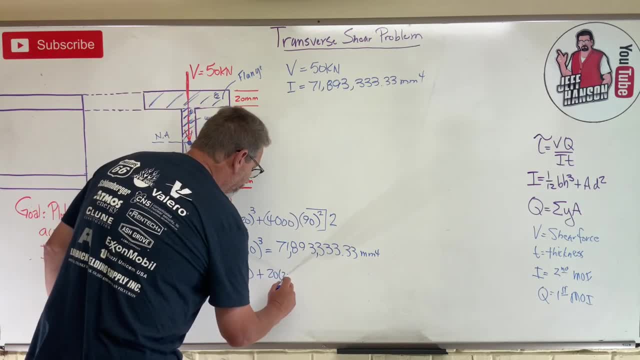 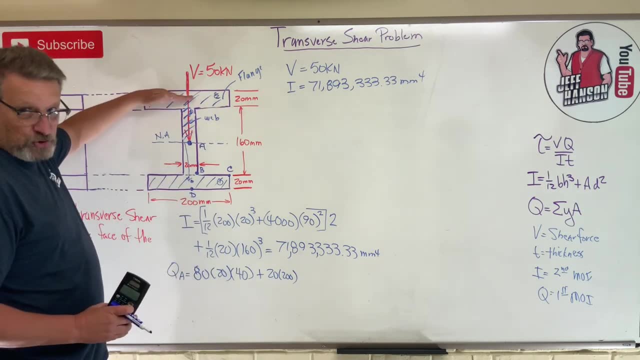 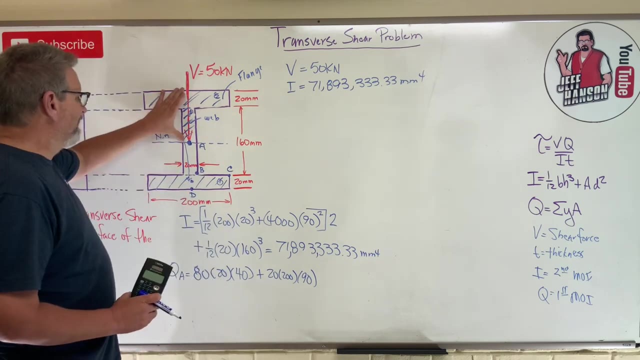 200.. That's the area, okay. And where is its centroid? I've got to go 80 and then I've got to go half of 20, which is under 10.. That's 90,, okay. And remember, I can just calculate a Q. 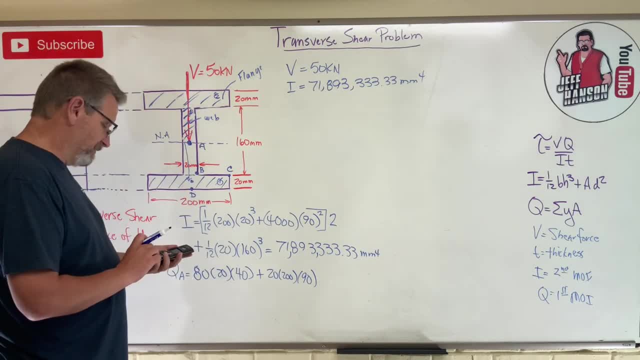 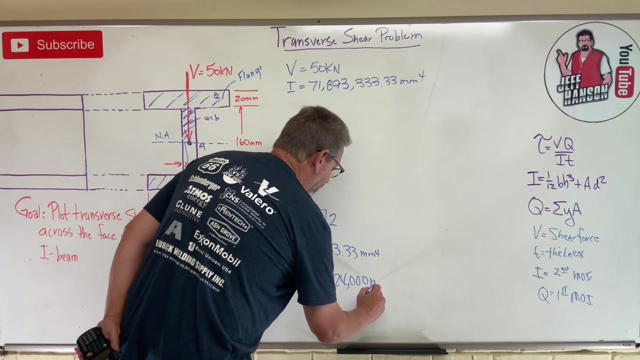 for the area below the neutral axis, I'll get the exact same number. Okay, so let's see what our number is here. It's going to be 80 times 20 times 40, plus 20 times 200 times 90,, 424,000.. Okay, that's millimeters cubed, but it's not a volume. 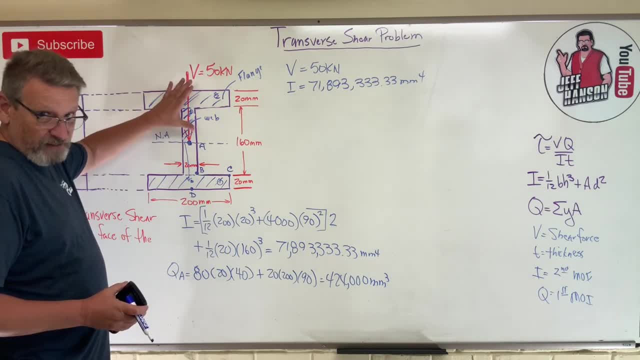 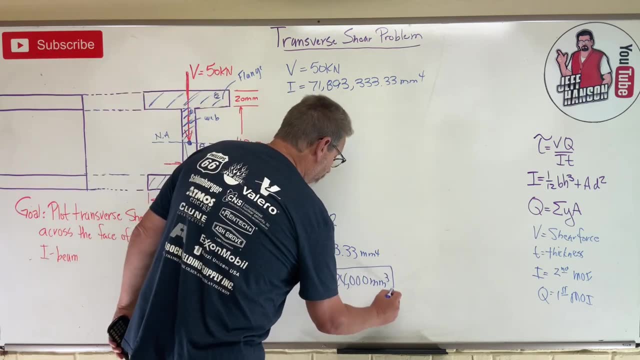 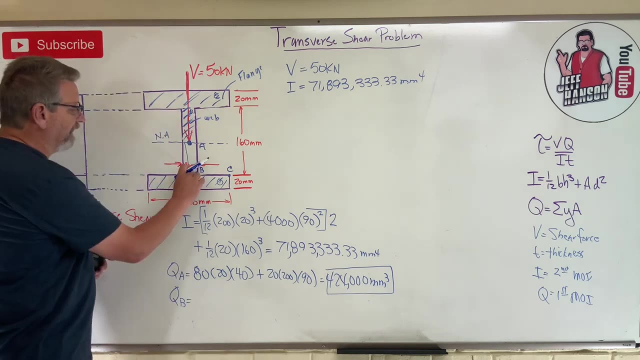 is it? Remember, it's a representation of where that area is above the shape times how far away that area is from the neutral axis. okay, So that is Q for point A. Let's do Q for point B while we're here, which is just going to be below point B. So it's just going. 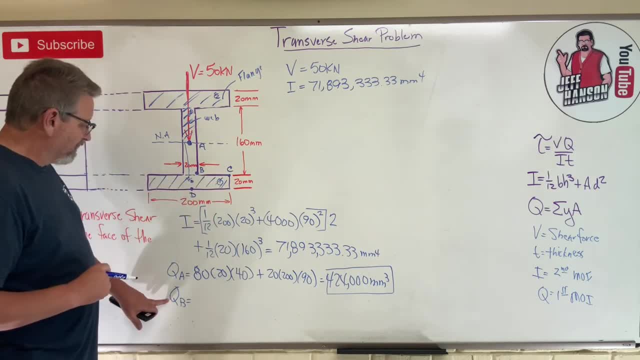 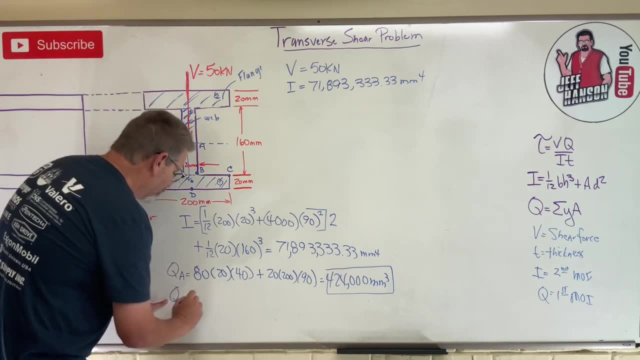 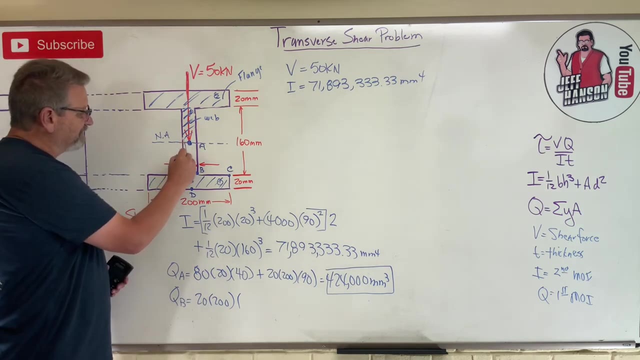 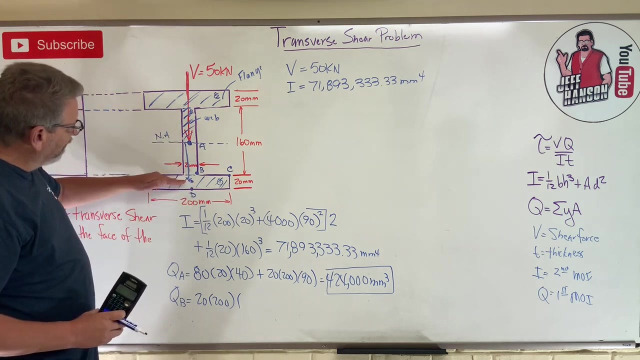 to be this little area down here. okay, So that Q is going to be that area. which is, how much is that area? Well, it's just 20 times 200, okay, Times the centroid, So the distance from the neutral axis down to the centroid of the piece part, which is 80 plus. 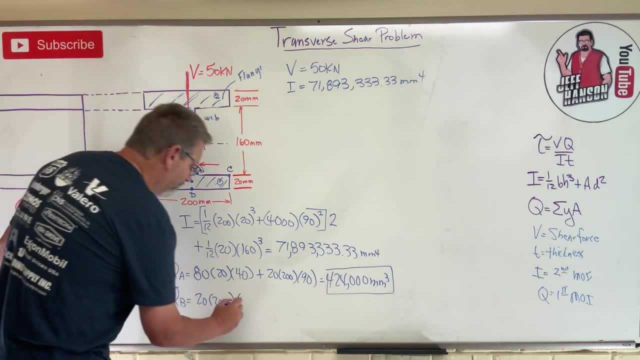 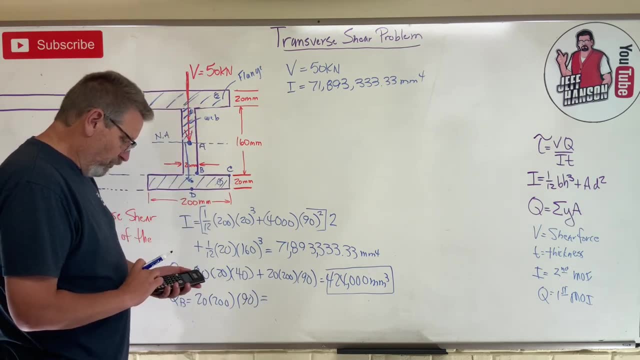 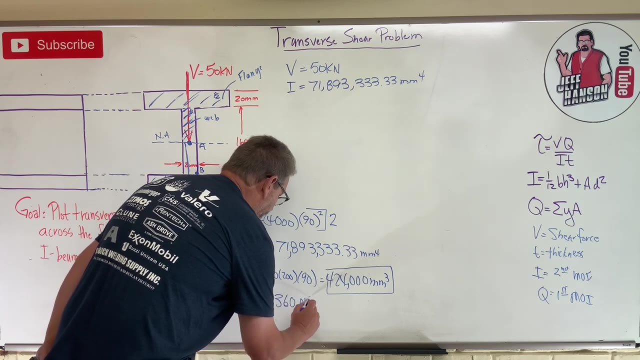 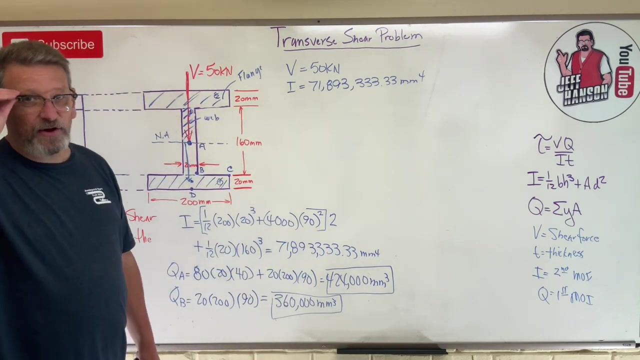 half of 20, which is 10 more, right? So that's 90,. okay, So Q for point B is 200 times 20 times 90,, 360,000.. Okay, I think we're ready to calculate tau here. okay, And for the 65th time, pay attention. 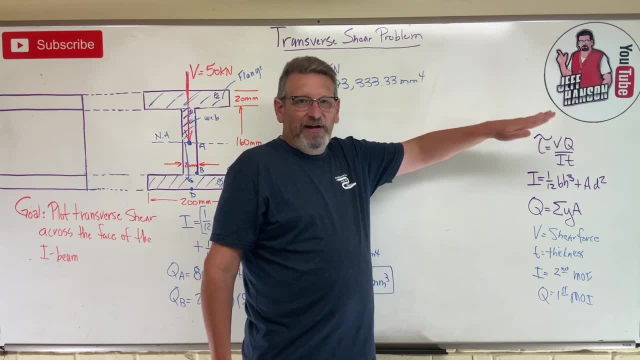 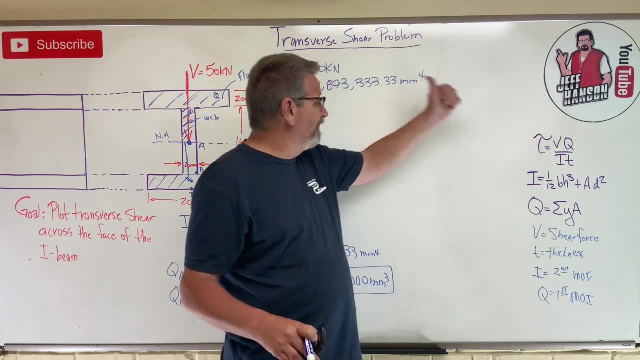 to your units. When you have a lot of things divided around here, we've got to have our units cancel out. So what are we looking for here for T? T is going to be in like PSI or KSI, but in the metric units that are working here we're going to try and get it in megapascals. 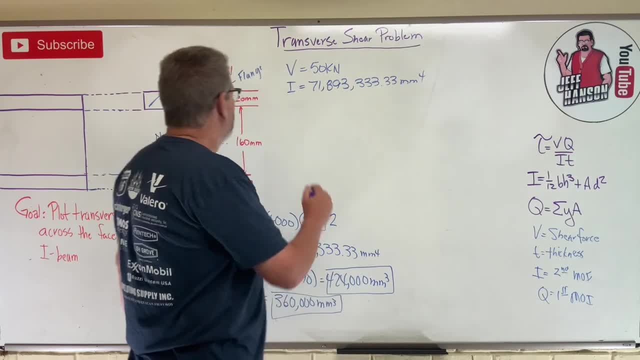 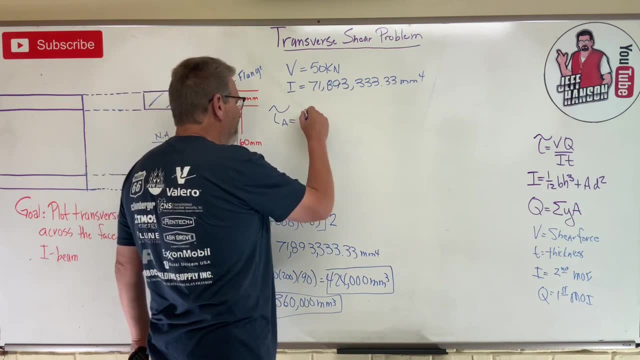 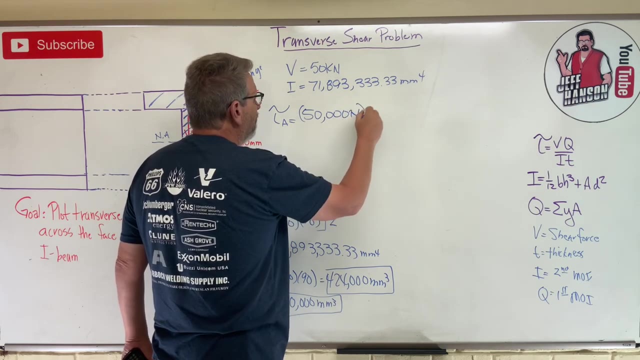 which is a newton, over a millimeter squared right. So here we go. So tau at point A is equal to V, which is given 50. And I'm going to put three zeros on here. okay, And that puts it into newtons, doesn't it Okay? Times Q for point A. Hey, we got. 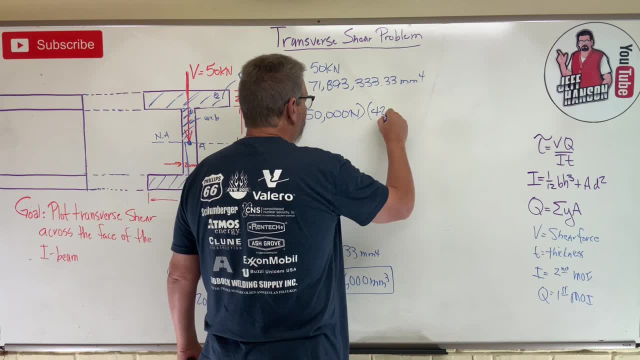 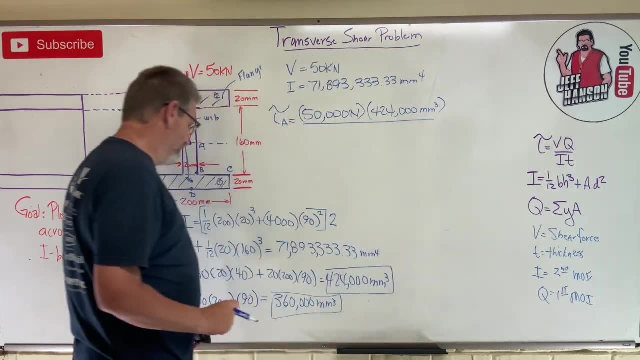 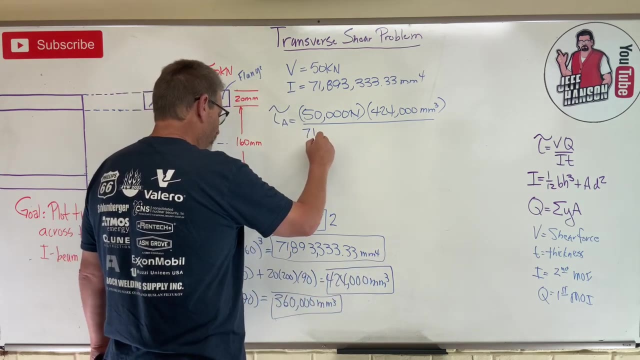 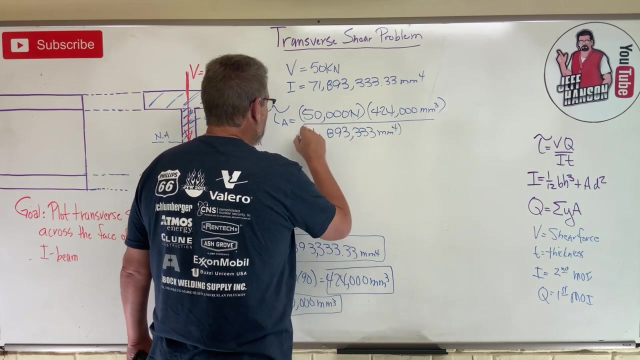 that too, don't we? 424.. And that's millimeters, cubed, okay, Divided by I. What is I? Here's I, this giant number right here, So scary 71,893,333, millimeters to the fourth times the thickness at point A, Okay point. 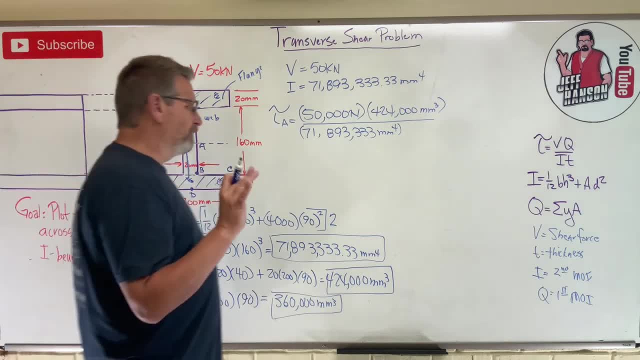 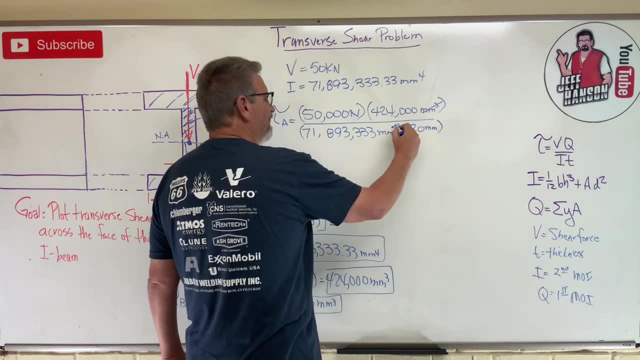 A is right here on the neutral axis, The thickness is only, it's only- 20, okay, M, M. So what do we got? There's three millimeters. That cancels that one out. So that's newtons over. 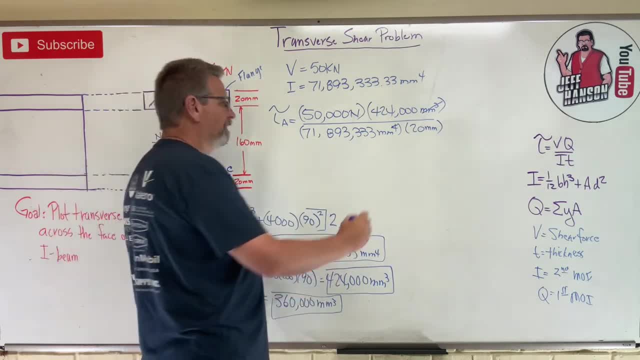 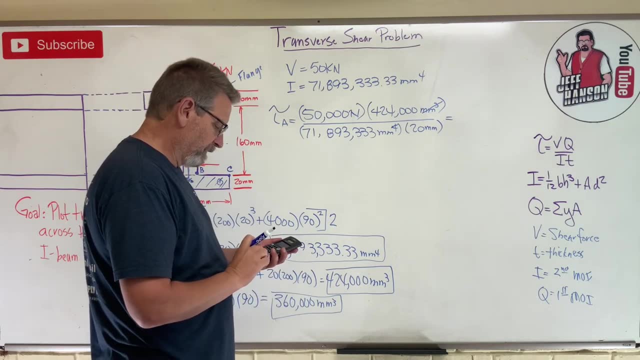 M, M, M, M, That's newtons over millimeters squared. Hey man, That's a megapascal. okay. So 50,000 times 424,000, equals. and then what? Divided by 20, equals. divided by a big number, 71,893,333, equals 14.74.. 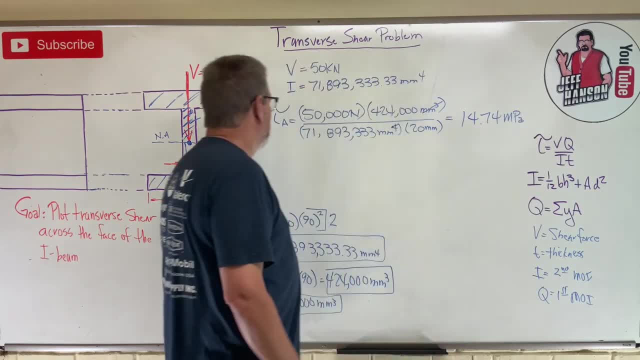 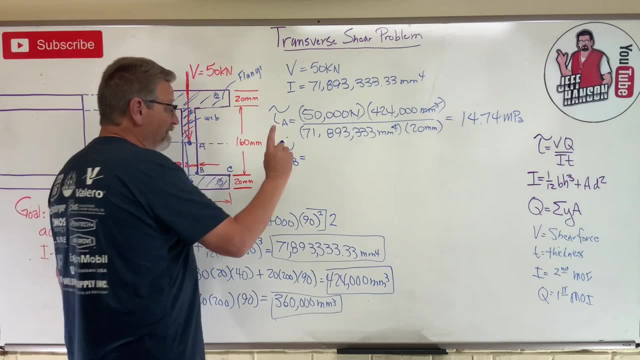 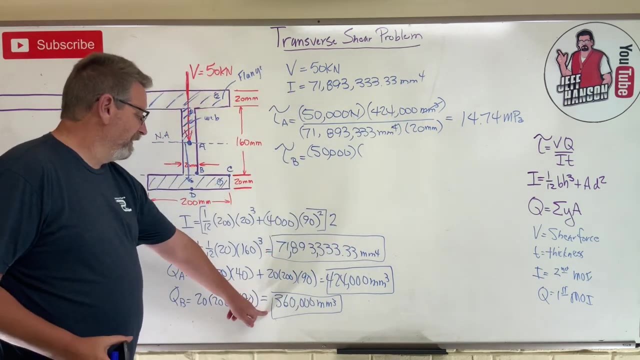 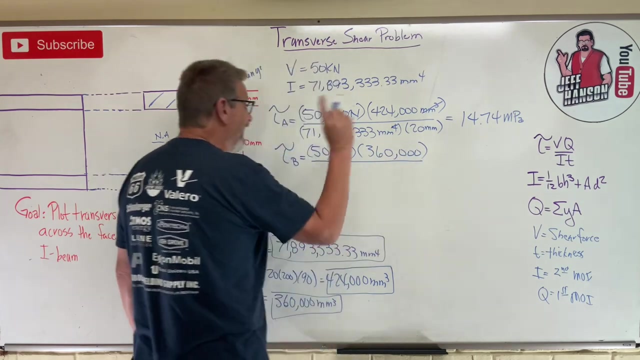 Okay, Genius, Let's do B. Okay, What is it at point B? Okay, Same shear force. Okay, Q, Q is different at B, isn't it? There it is. We found that guy, 360,000.. I is the same. 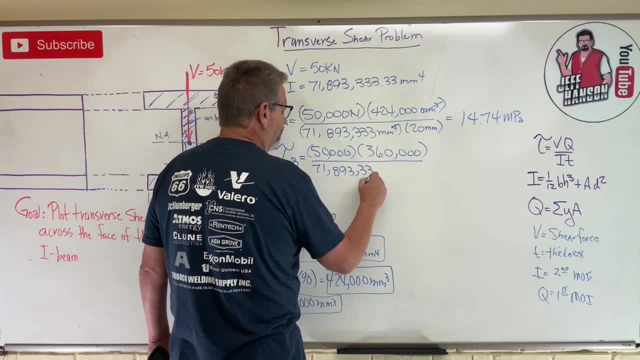 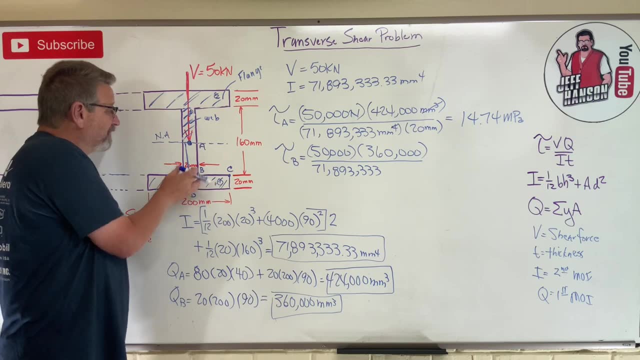 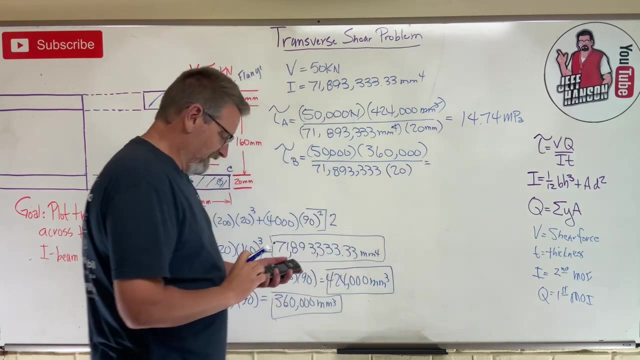 71,893,333.. And you know what? The thickness at point B, which is one molecule into the flange or the web- rather right, It's in the web- is still 20.. Okay, So let's see what that is. 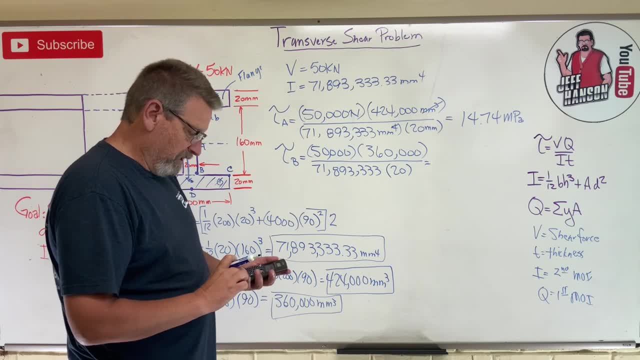 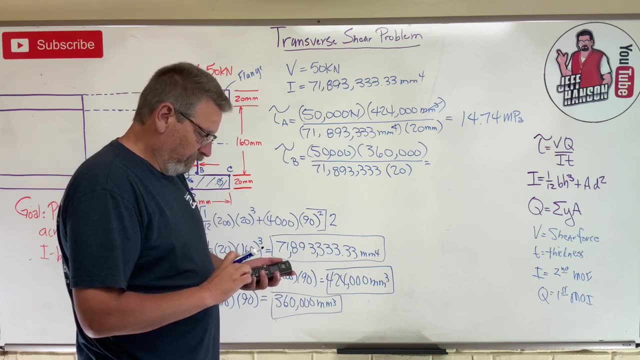 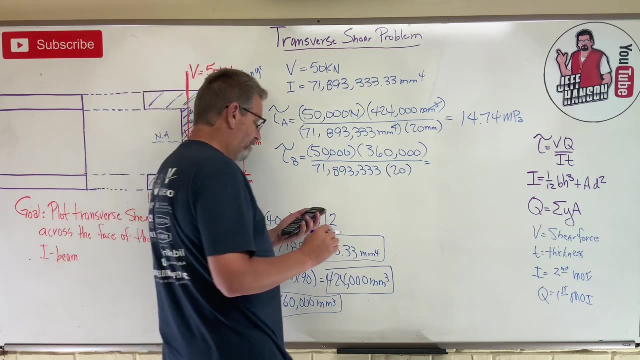 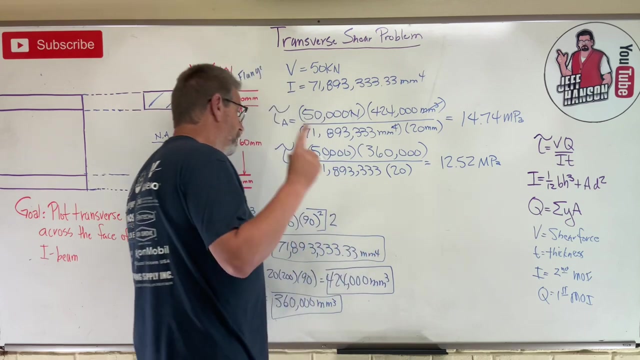 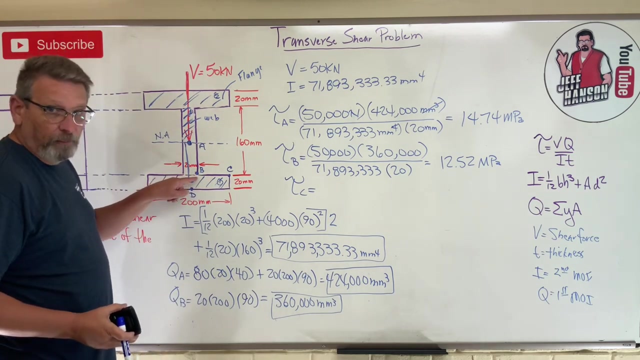 50,000 times 360,000. equals divided by 20, equals divided by 71,893,123, equals 12.52.. All right, A couple more. Let's do C. Okay Now. C, remember, is one molecule below point B, So C. 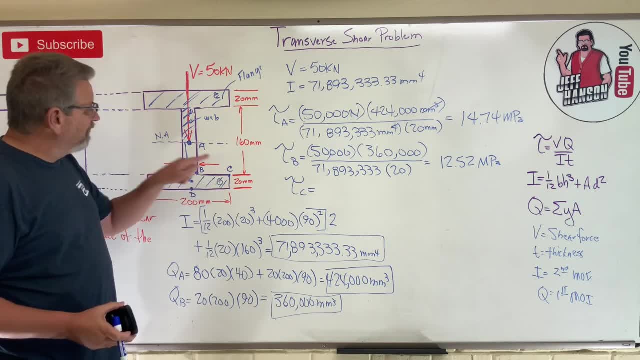 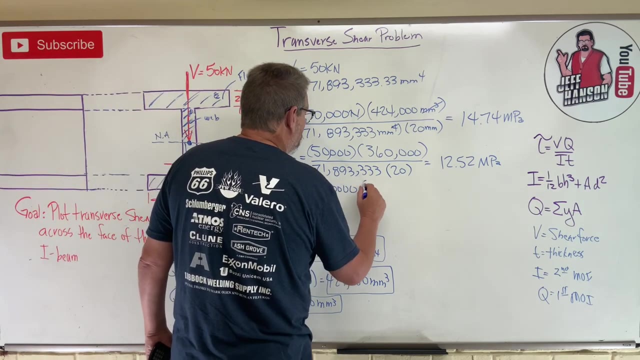 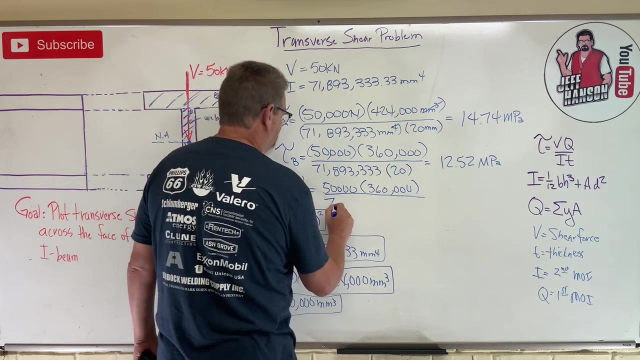 is into the flange. Okay. So what's going to be different about the equation for B? Is Q going to be the same? Yes, There's still the same amount of area below C as there is below B, So that's the same. So I've got 50,000 times 360,000, divided by I, I is always the same- 71,893,333.. 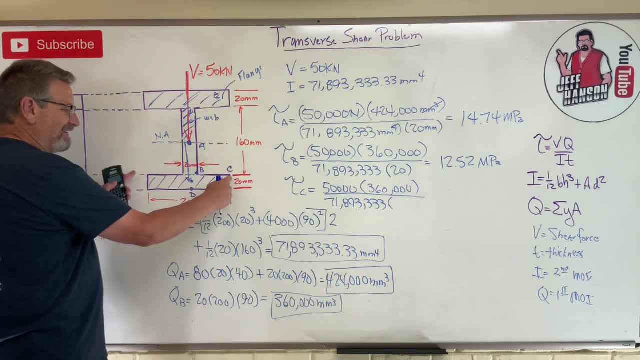 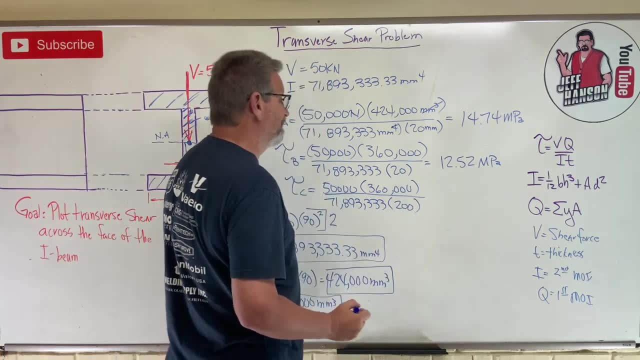 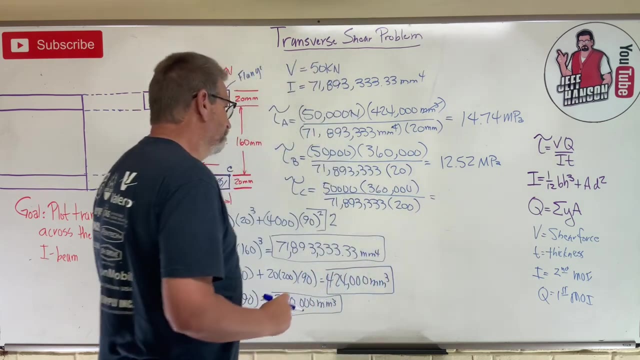 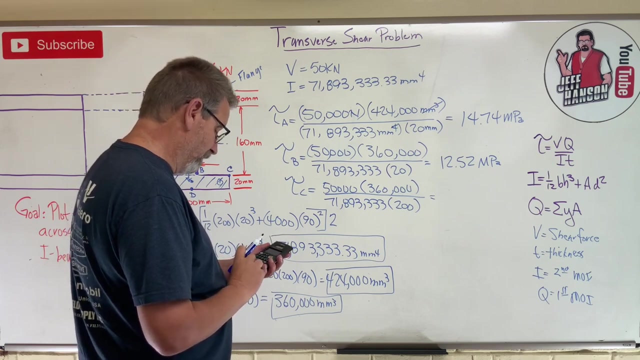 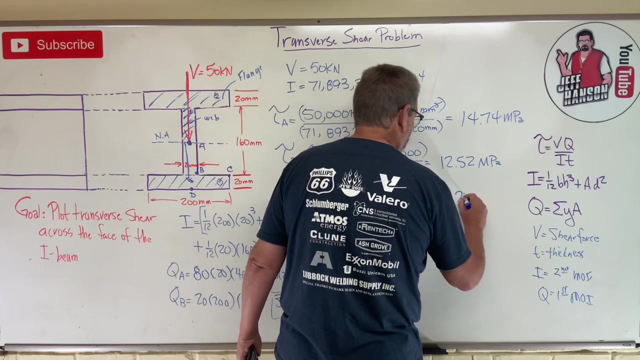 Now, what's the thickness of the beam at point C? Now it's 200.. Okay, 200.. You know what that's going to do? That's going to move that decimal over one place, isn't it Right? So I can take that 12.52, and multiply by 20, and then divide by 200. It's a 1.25.. Okay. 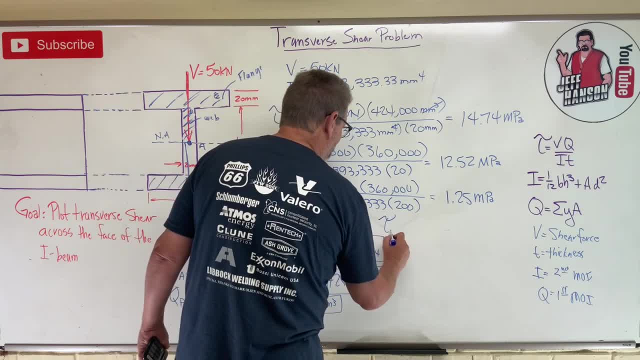 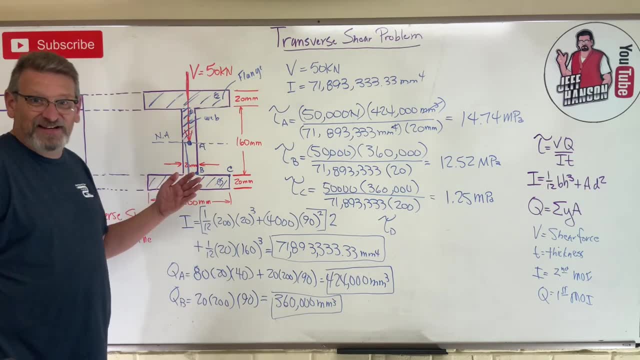 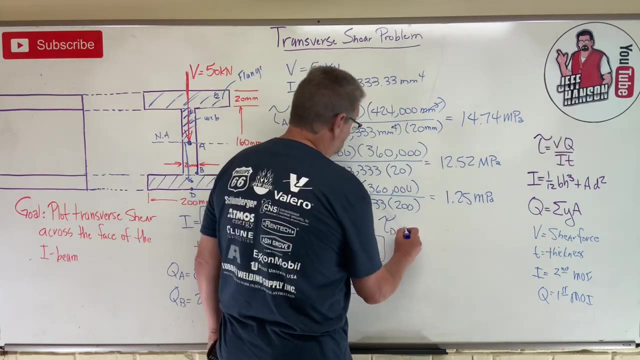 One more, Last one: Tau at point D. Okay, How much area is below point D? Point D is on the outside of the part, None. What happens when Q is zero? How much is the else tau equal to Zero? All right, now I think we've got enough information to. 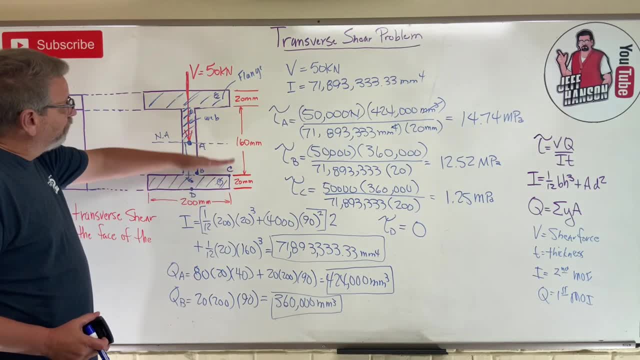 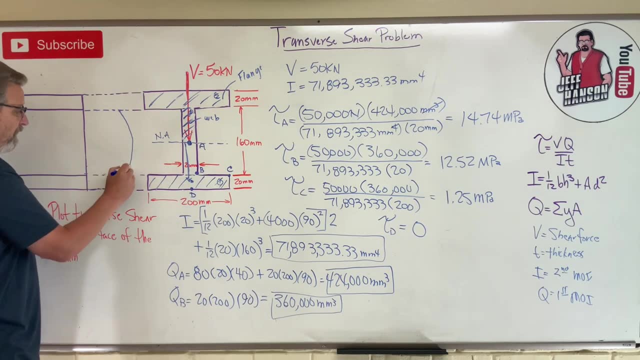 plot this Now. I only work parts below the neutral axis, but I know this is symmetric and there's gonna be the same thing above it, isn't it? Okay, so my graph is gonna look something like this: Okay, so at this point, here is the max. 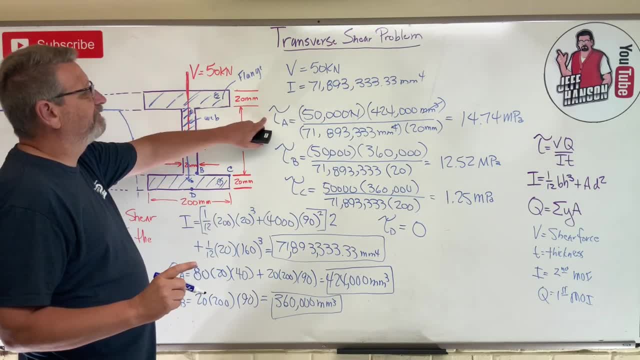 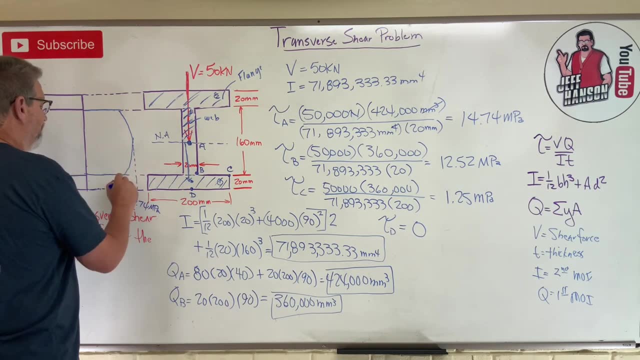 remember, the maximum shear stress always happens at the neutral axis: 14.74 MPAs, okay, and then down here, you know slightly less, 12.52 MPAs, and then I got this big jump and then down at the bottom, I got these little guys down here. 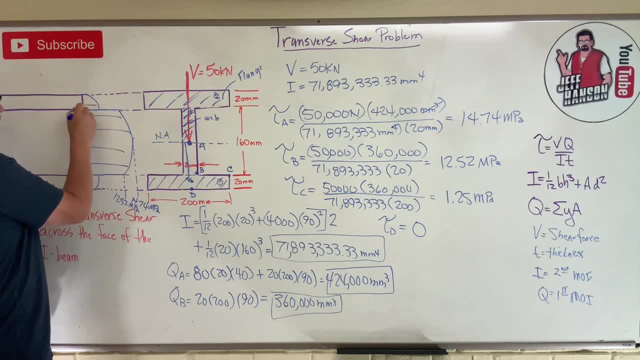 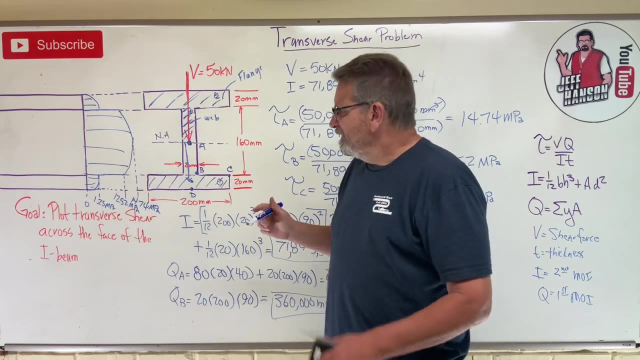 right, because the thickness jumped right, because the thickness jumped over. here it's found 1.25.. And, of course, down here, at the outside of the part, the shear stress goes to zero. Now I'm going to tell you: the shear stress is maximum at the neutral axis and zero at the. 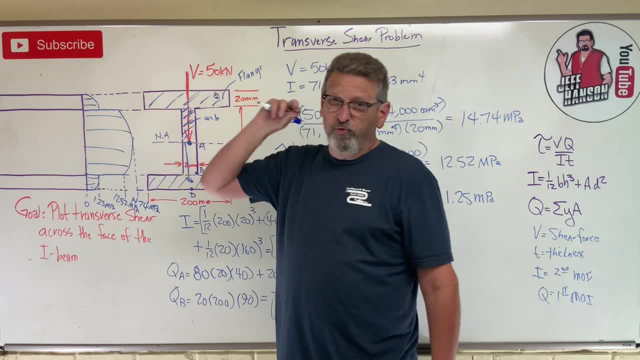 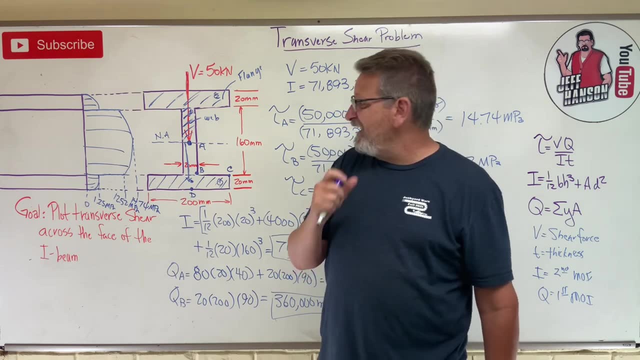 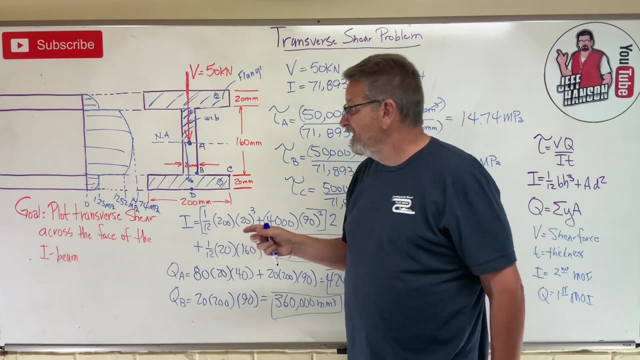 outside And I want to say always, there are some really weird geometry beams that have a super thick at the neutral axis that when you divide that out the maximum shear doesn't wind up being at the neutral axis. But that's like about 0.1% of the beams that exist in the world For the